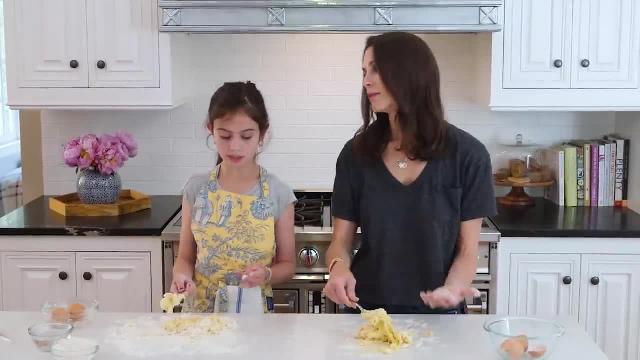 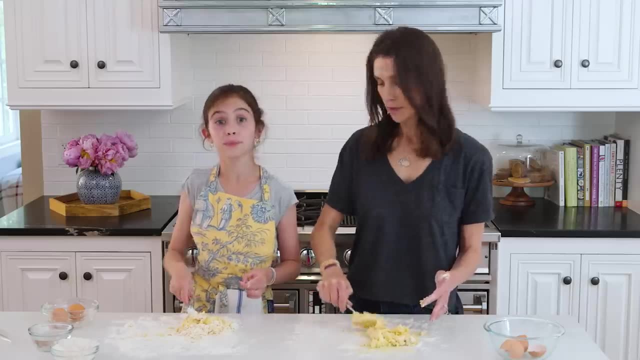 is: you need more water? Well, because sometimes the egg is bigger. so that depends on everything. The eggs aren't perfect size, right? They're not all the same size, or else the world would just be weird. And now, actually, we're gonna start using our hands. 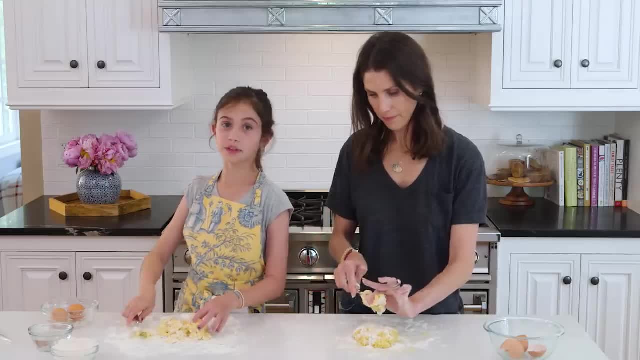 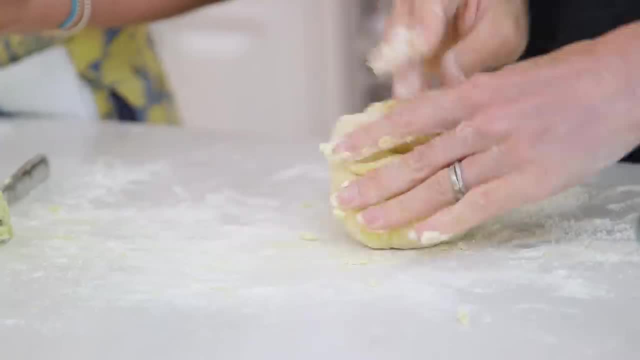 The moment. I've been waiting for Every chef's favorite tool, And then when it's getting tough, like really tough to do this, you know it's time to go back. Oh, that's how you know. okay, That's what I was looking for- a little hint. 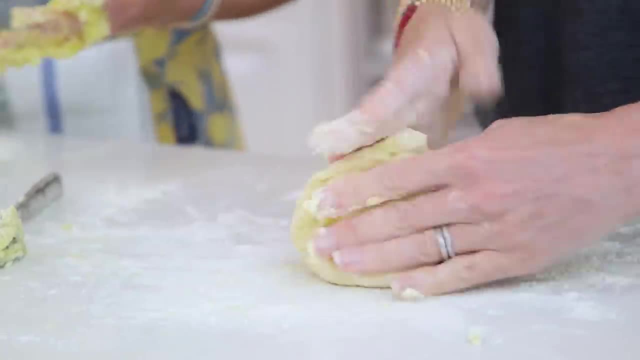 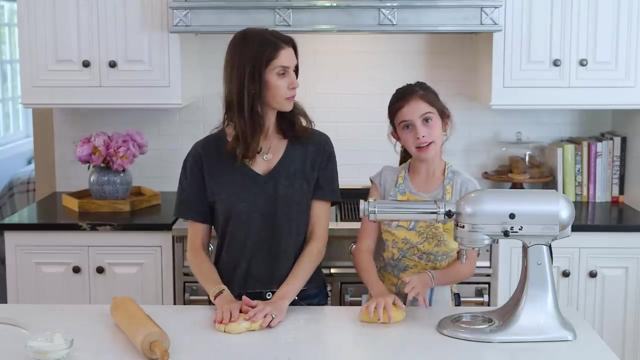 You go like this and then I fold it over. Yeah, Got it. Okay. so I think my dough's about ready, Our dough is done, so now we are going to thin it out. I gave my mom the hard job which is with a rolling pin. 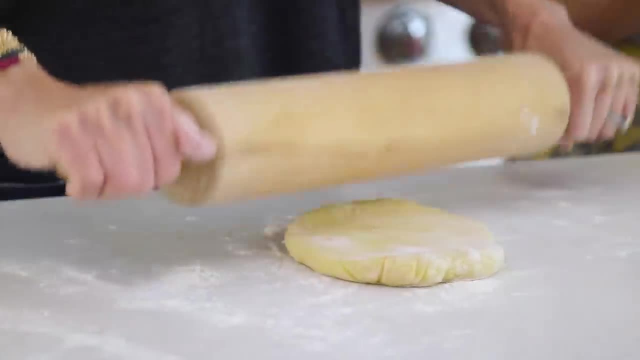 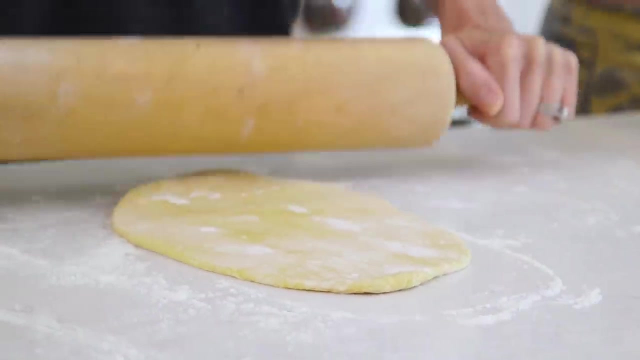 All right, okay, And we cleaned our surface off too, guys, so it wouldn't be all sticky. Okay. Yeah, Is this good? No, not at all. Not at all. You saw how thin it has to be and how long. 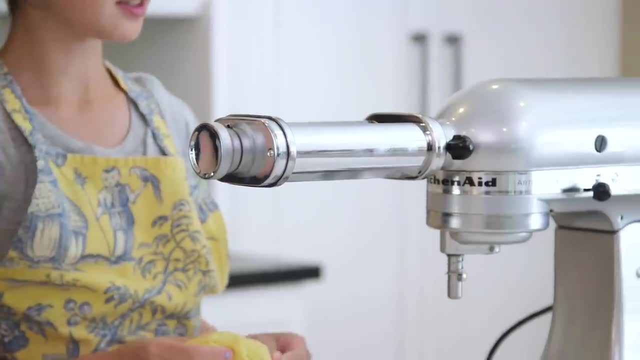 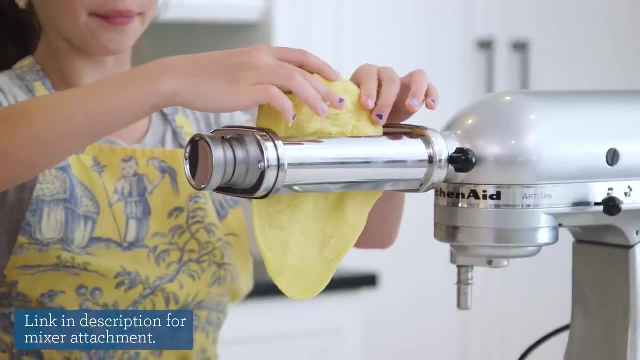 So okay, so you're using a pasta attachment for a mixer, Yeah, Okay, First you have to set it to one, So I'm just going to put it in. That's like the widest setting. Yeah, That is so cool and so much easier. 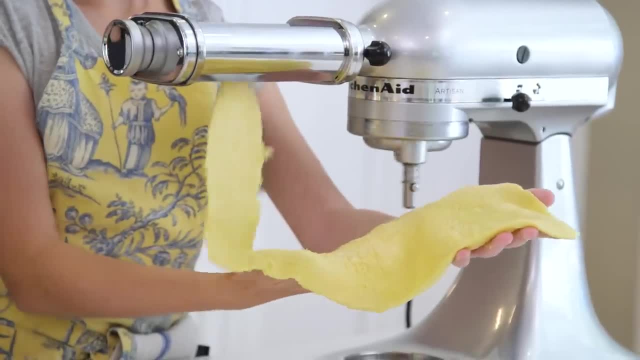 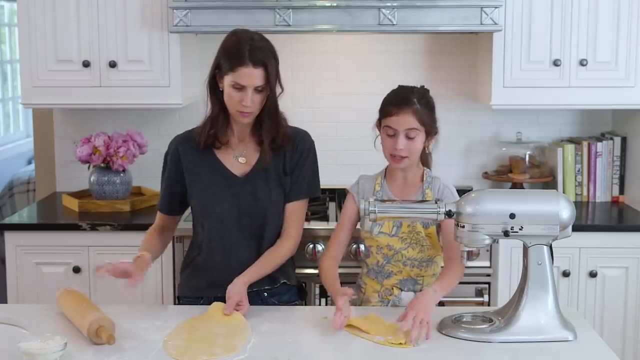 I definitely got the harder job. Yeah, It's a little sticky, so we're going to add some flour, All right. And then Mom does a lot of flour. Then you have to fold it, no matter what. Okay, do I need to fold mine, or can I just keep going? 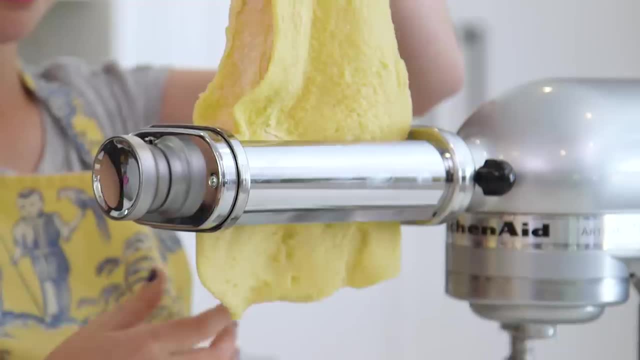 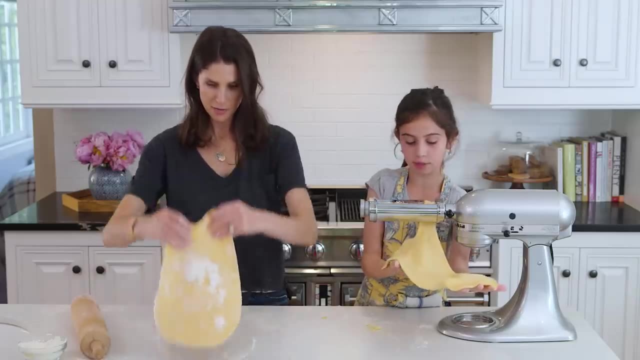 No, you have to keep on going. You're not folding it, And then I'm going to put it back through. Don't mind me, I'm just still rolling over here. Oh, that's actually pretty good, Mom. Pretty good right. 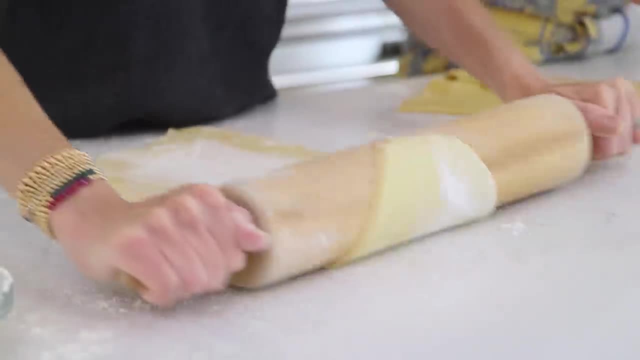 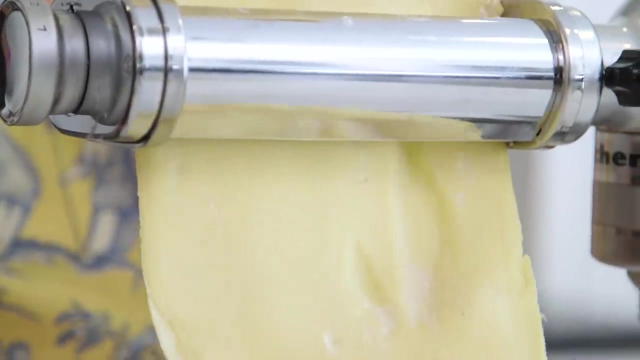 Yeah, I'm feeling good about myself. You should be. I'm going to turn it to two. Two, Okay, so we're making it thinner now. right Now, you went to two. How far up do you go? Because there's eight on here. 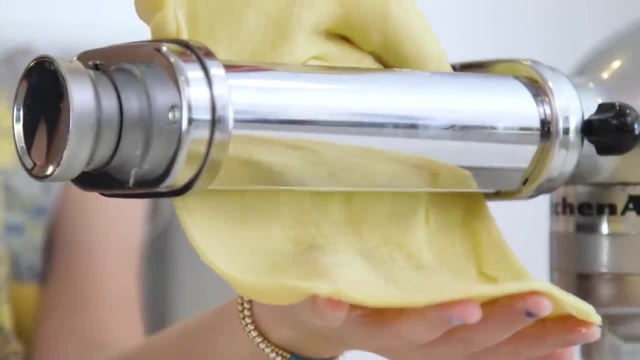 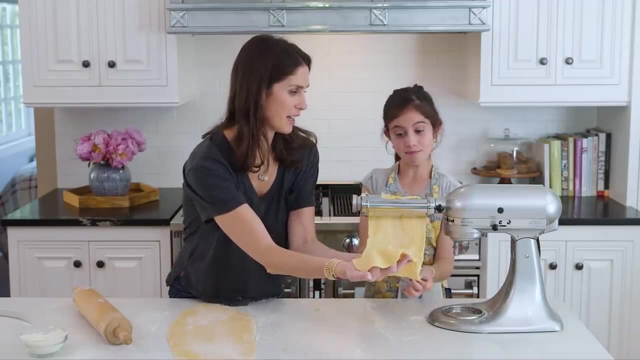 Okay, so you go to five of eight. How many times do you put it through? each one? like twice, Oh, yeah, Okay, And You just need like multiple hands catching it. You want my help? Maybe a little, but, Mom, you need some work too. 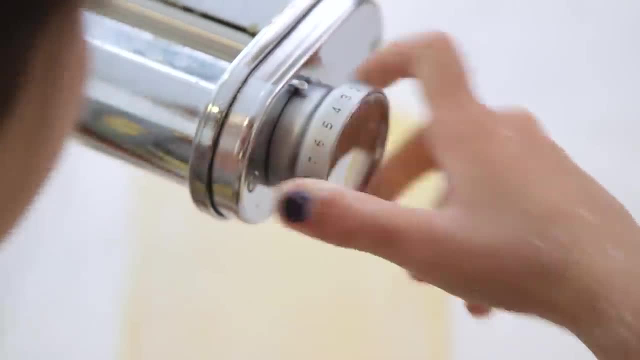 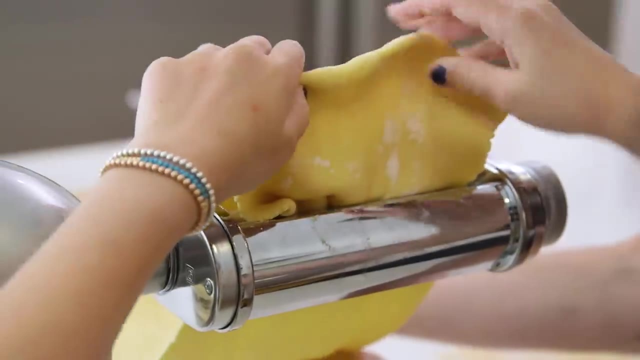 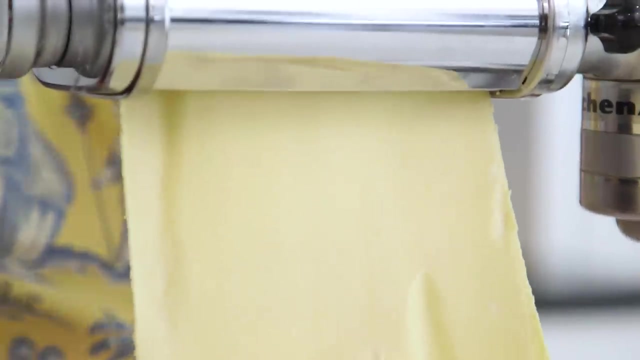 I still need work Now. I'm just going to go up to three. Woo-hoo, We're going to pop it and go to five. See, it's kind of like smooth and pretty. It's really awesome. I can't believe how much the texture has changed. 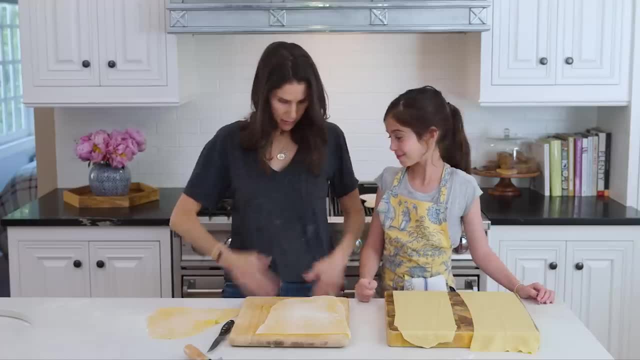 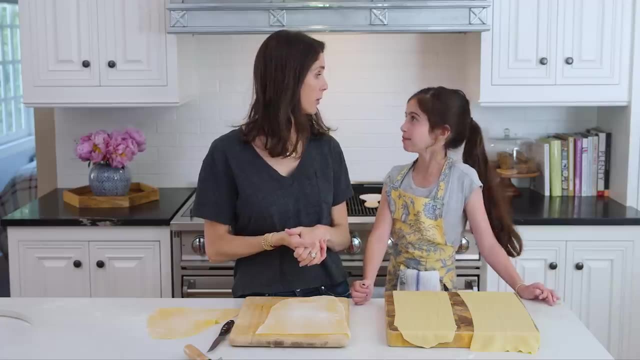 Yeah, And we're done. Should have worn an apron. All right, what's next? So now, our dough is done, So we are going to make our shape. What shape are we making? A bow, Bow, butterfly. 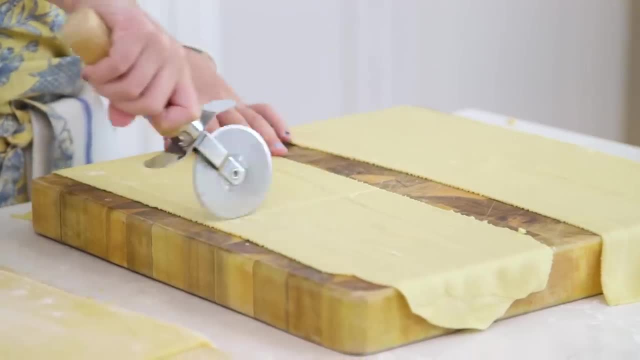 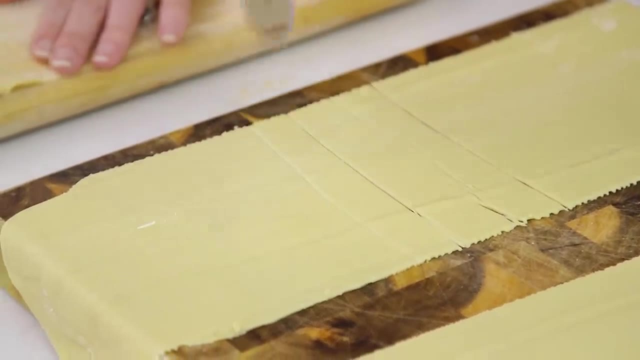 What are they called in Italian Farfalle? What do we do? Oh, Avery's using the pizza cutter again, with the easy way: Basically, just make strips like this. So how thick? Like an inch thick? Yeah, Okay, an inch thick. 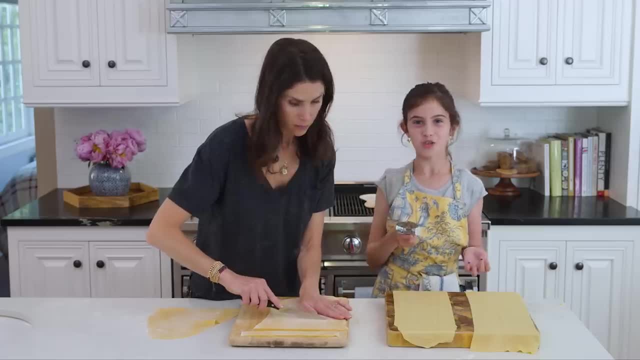 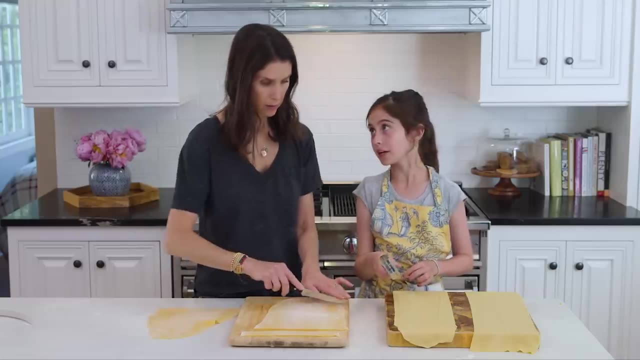 You could even make for this you can make your bow ties into like a fun, strange way. Mm, I wonder how you do like corkscrew pasta or like fusilli or something. Yeah, It's probably a lot more complicated. 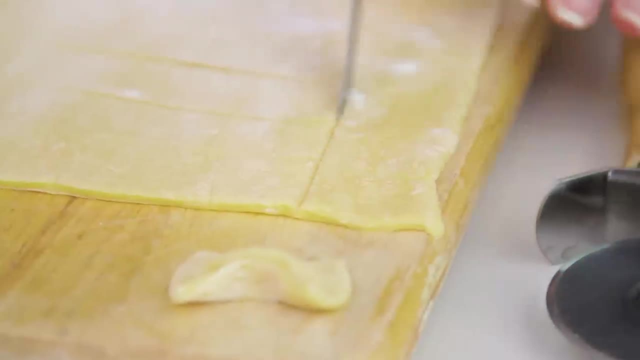 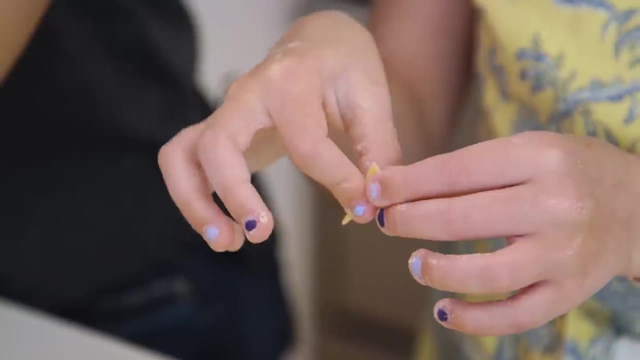 Yeah, probably. Next you're going to cut a rectangle, Okay, And then you're just going to go like this. It's so hard to make. I think that was sarcasm. It was: Okay, I'm just, you're just pinching it. 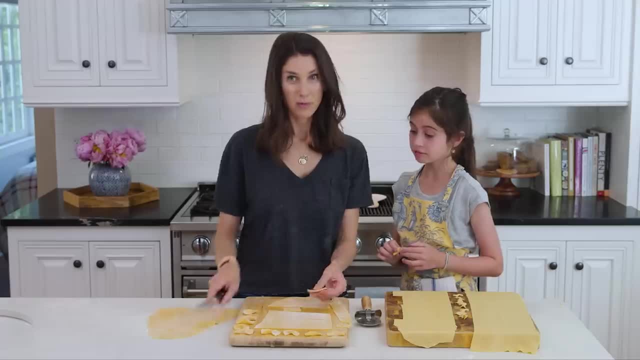 Yeah, I think this will be enough for Brooks and Ryder for dinner tonight. I know They seem pretty hungry, Yeah, but then the thing that works. Wait, what about me and Daddy? We don't get any, Woo-hoo. 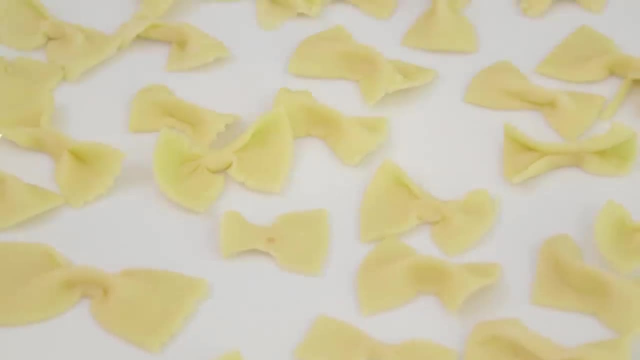 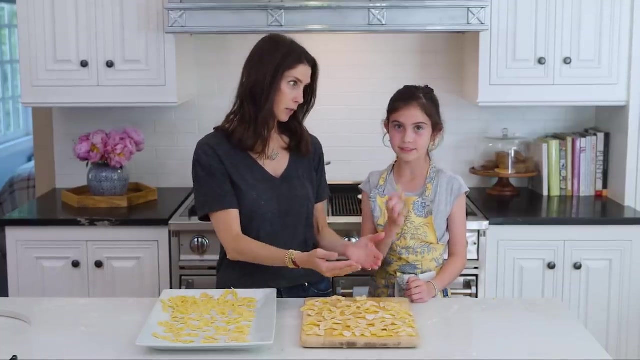 Okay, so we got our pasta all ready. Ta-da, Mom's got the water boiling And now we got to cook it. Now, cooking time does vary, right? Yes, It can be thicker, Like these guys. It can be longer, right. 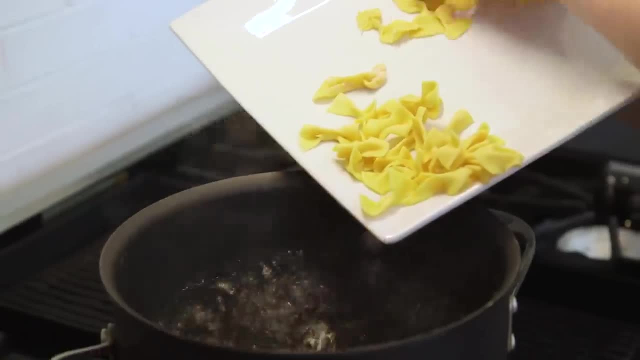 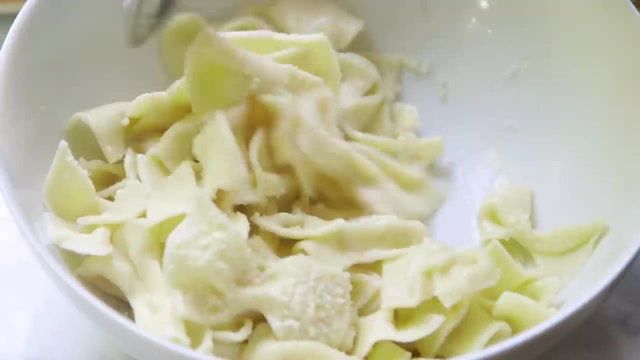 So anywhere, I would say from like 3 to 10 minutes when we were experimenting. that's about right. Yeah, Mm-hmm, Okay, All right, the pasta is off of the stove and it smells amazing. Yeah. 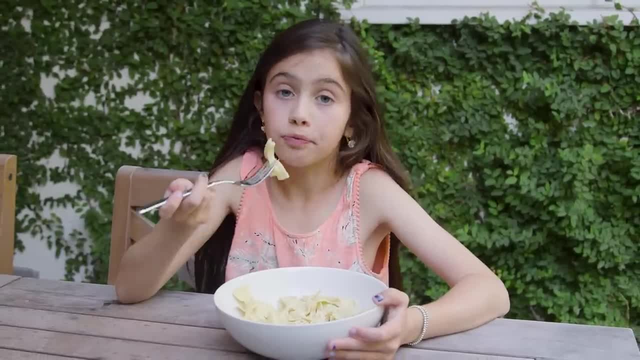 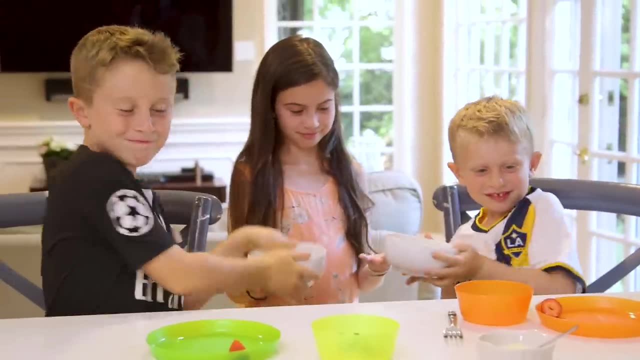 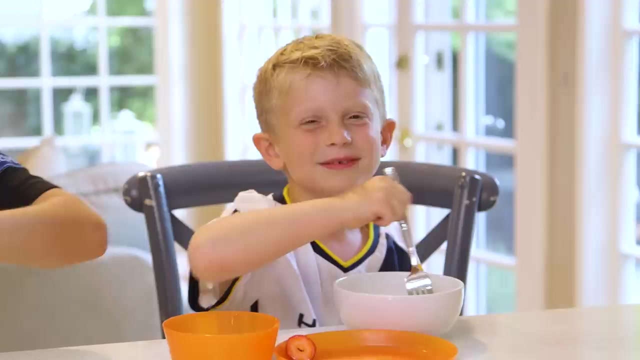 Cheesy, buttery, even better than sherbet. Should we have the boys try it? Definitely: Pasta, pasta, pasta, Mmm, Thank you. I mean this is delicious. This is better than the stuff that Mom buys. 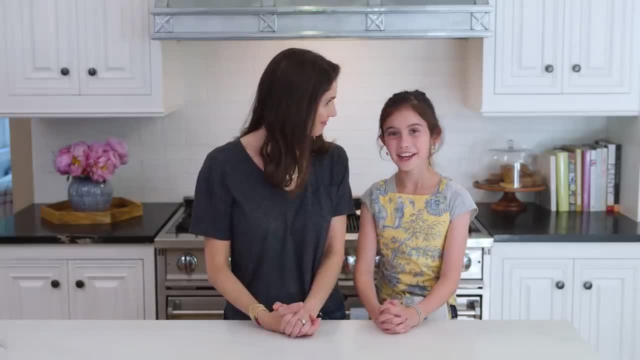 All right. well, that wraps up our pasta episode. Thank you so much for showing me how it's done. If you liked this episode, stay tuned, Because next time we're doing Sauces and ravioli. All right time to mangia. 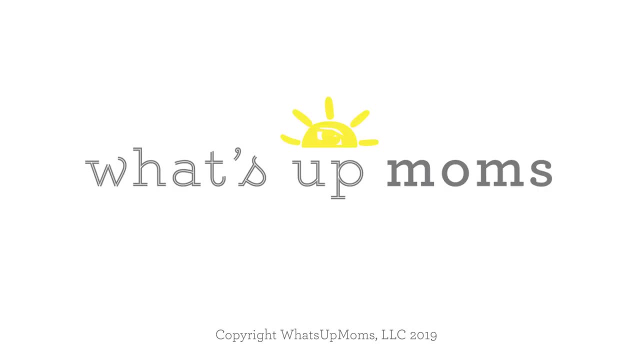 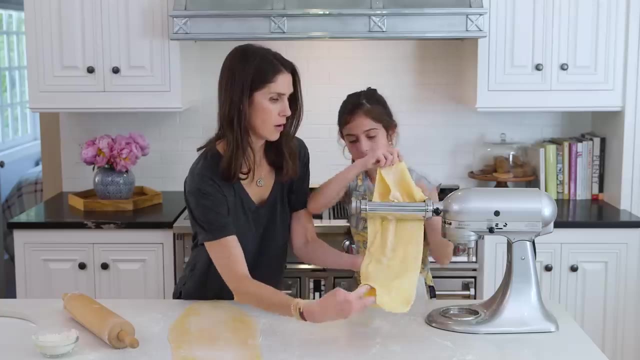 Bye guys. Itali, Two, three action. You're going to see that. Oh, Just go into that. Oh There, No, Oh well, And we're just going to cut them up and you'll see.